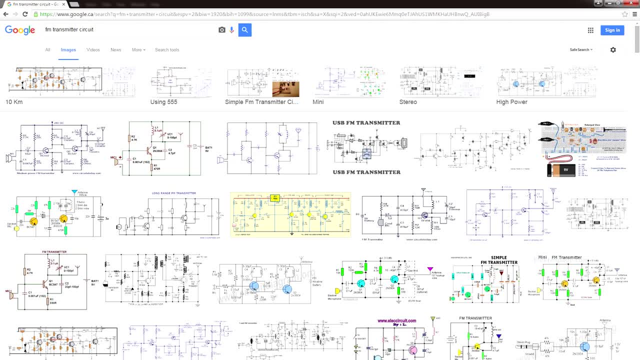 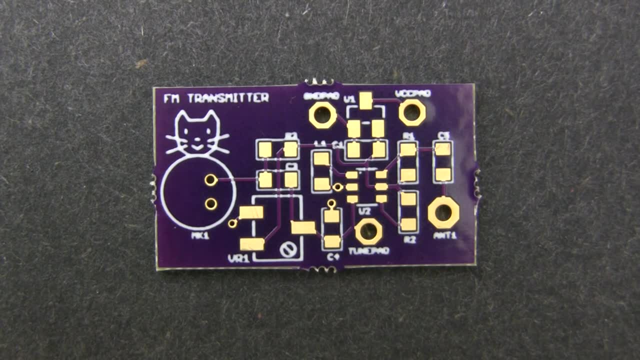 And there are many others. There are many FM transmitter circuits out there, but in my experience most of them are very unstable, so I made my own. This circuit requires a PCB and I got mine from OSH Park. It cost me $3 for three of them, including shipping. 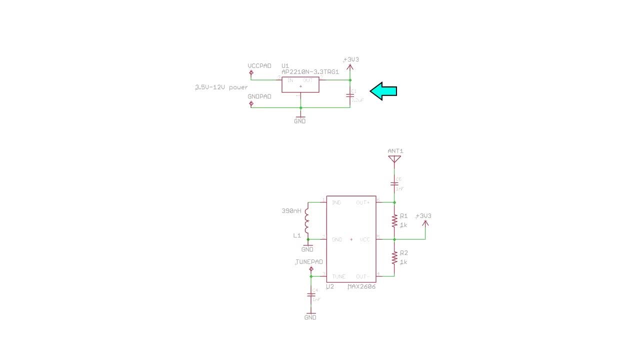 and I'll put a link in the video description section. The first part of the circuit is just a 3.3 volt linear regulator to create a nice stable 3.3 volt supply. The main part of the circuit is a Max 2606 Voltage Controlled Oscillator IC. 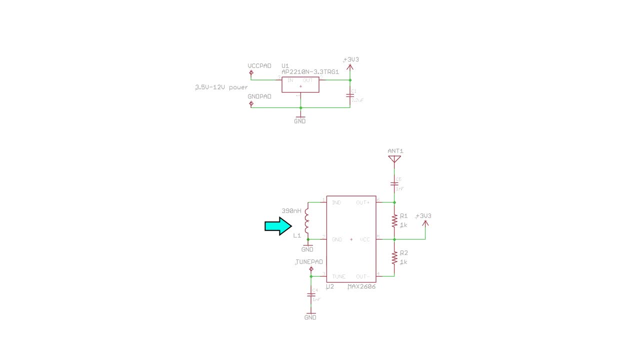 This inductor sets the approximate frequency range that the Max 2606 will oscillate at. If you read the datasheet, you'll see that this chip can oscillate from 70 to 150 MHz, and we just want it to put out roughly 100 MHz for the FM band. 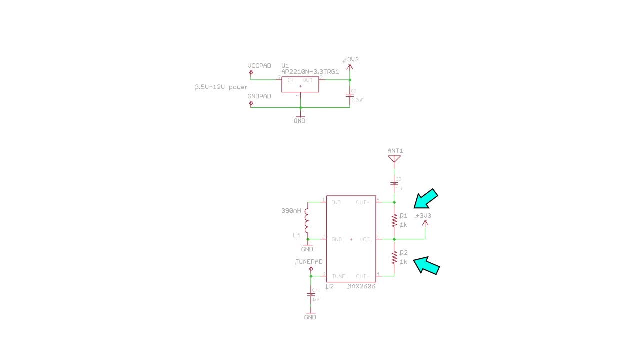 390 nanohenries takes care of that. There's actually a small amplifier inside this oscillator chip and these resistors form part of it. I want you to know that this isn't the optimal way to set up a radio amplifier. I'm just showing you something that's low powered. 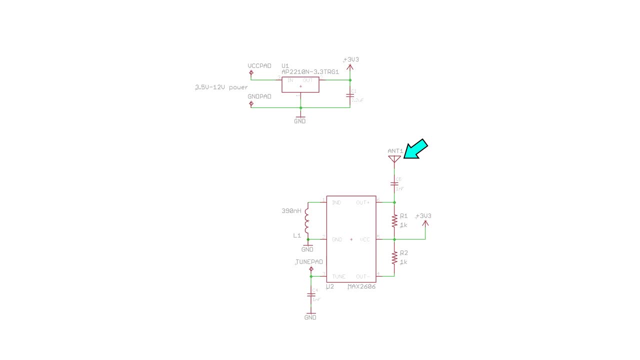 and will work across a wide range of frequencies. For the antenna you can just use a piece of wood. You can also use wire about a meter long, but only add it after you're done testing things. This capacitor forms a high pass filter to make sure that no DC voltages can. 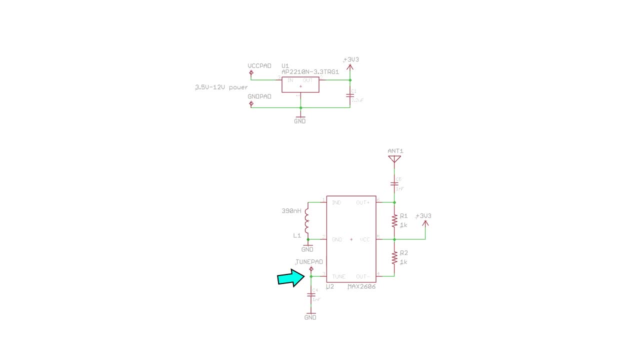 accidentally reach the oscillator. Now this pin, the tuning pin, is where the fun starts. By applying a voltage here, we can control the exact frequency that the oscillator spits out. So let's do that. Let's add a simple potentiometer voltage divider circuit to apply an adjustable DC voltage to the tuning pin. 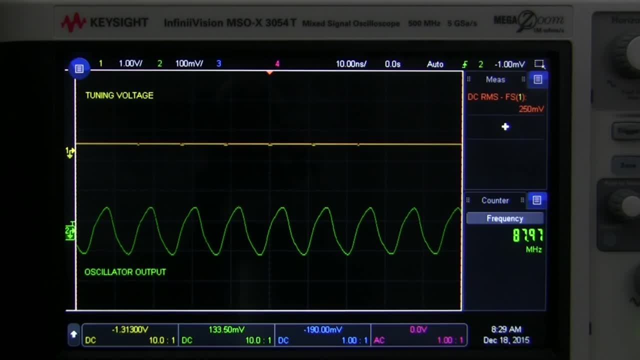 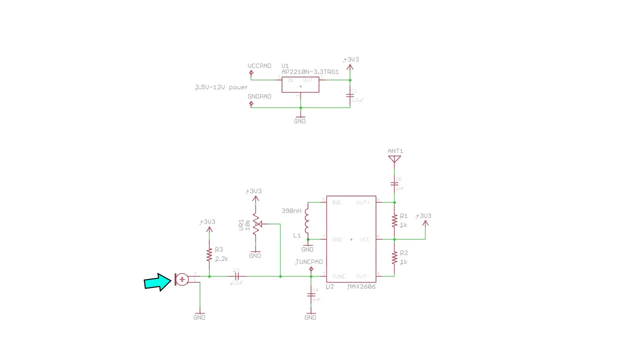 We can change the voltage at the tuning pin which controls the oscillation frequency, And we can choose pretty much any frequency in the consumer FM radio band. Now let's add a microphone. It's the same basic microphone circuit you've seen in many of my videos before. 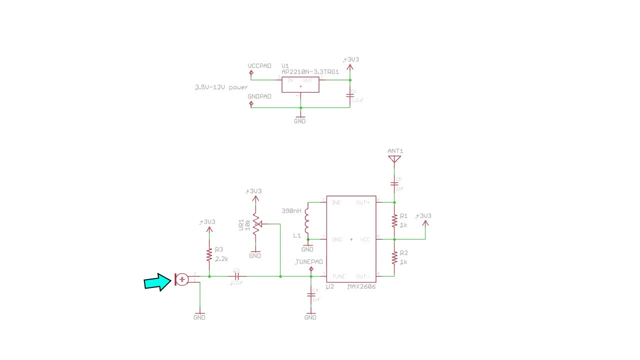 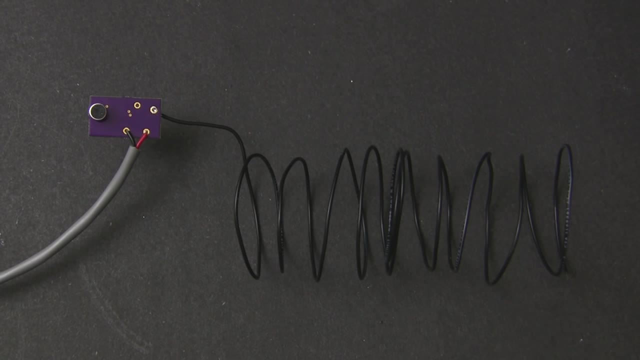 This will add a tiny millivolt level voltage swing on top of the larger DC tuning voltage. This will modulate our carrier wave just enough to carry audio. Let's add a microphone onto the bottom side of the PCB and add your antenna. Now set your FM radio to a blank station and use. 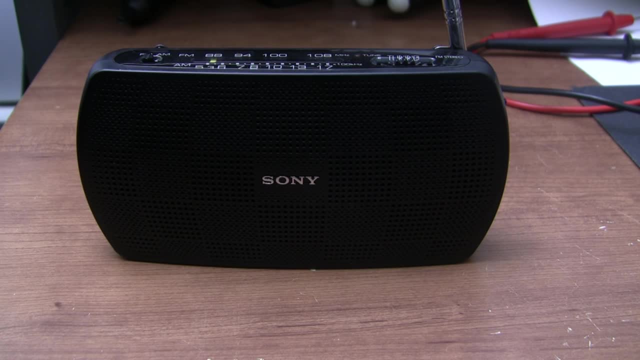 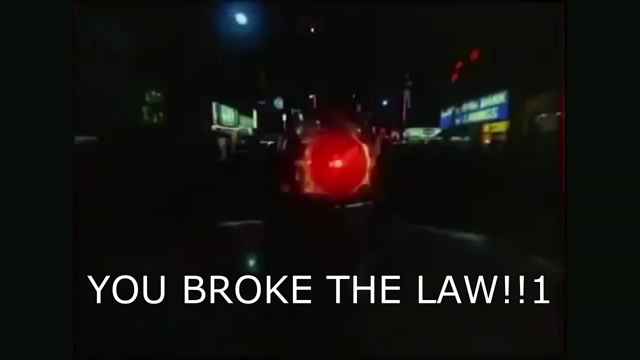 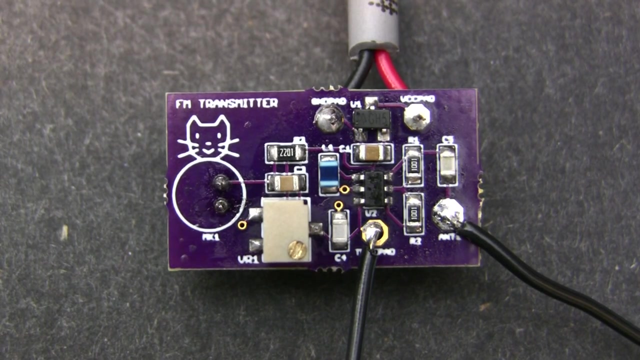 the potentiometer to adjust the frequency of your transmitter until you hear silence. And that's it. your FM transmitter is complete. Actually, I didn't. This design is low powered enough that it's legal to use in almost every country. However, what's absolutely not legal anywhere is